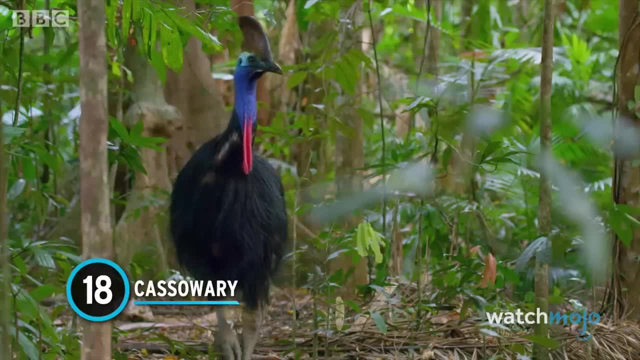 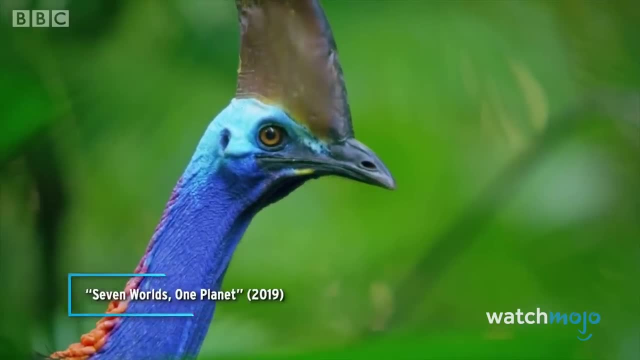 Number 18. Cassowary: If you're looking for proof that birds are related to dinosaurs, look no further than the cassowary. Armed with powerful legs and dagger-like claws, the cassowary can deliver a kick that will break bones and slice through flesh. Number 18. Cassowary: If you're looking for proof that birds are related to dinosaurs, look no further than the cassowary. Armed with powerful legs and dagger-like claws, the cassowary can deliver a kick that will break bones and slice through flesh. 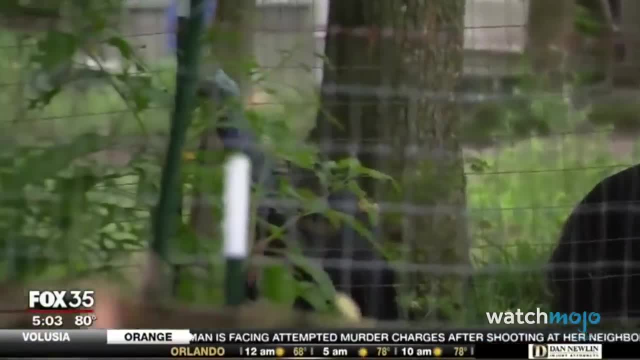 Number 18. Cassowary: If you're looking for proof that birds are related to dinosaurs, look no further than the cassowary. While these large birds are cautious around humans, more than 100 instances of people being attacked by cassowaries have been reported, most of which involved food. 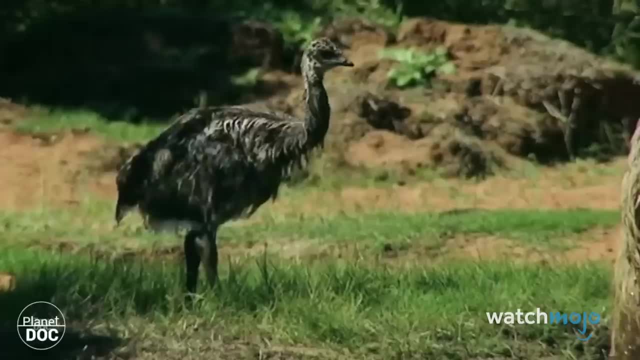 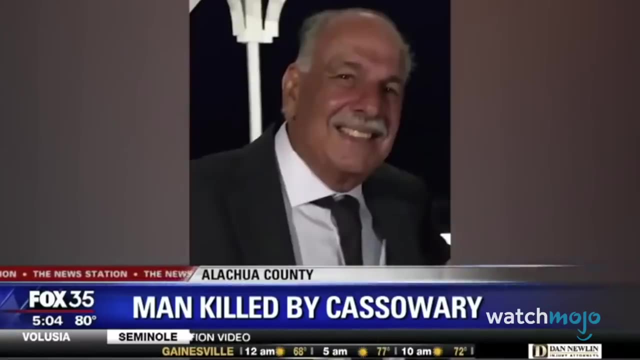 Thankfully, fatalities are rare. Though it's possible for the cassowary to be partially domesticated, owning one can still be dangerous. In April 2019, a Florida man was killed by a cassowary he raised when it fatally injured him after he fell down. 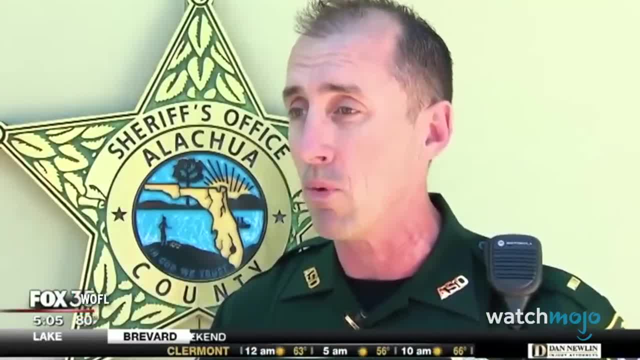 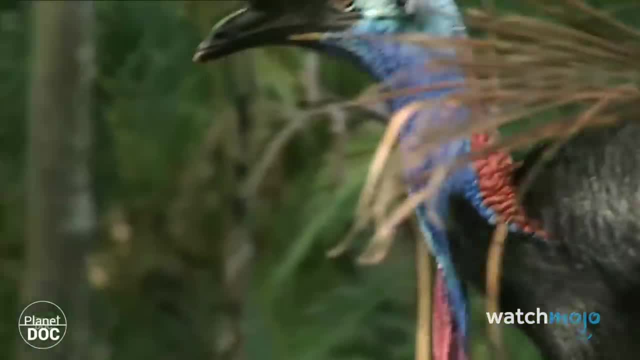 We believe he went in there to recover that egg and then at some point the bird was able to to make its attack. The cassowary's potential for harm has earned it the title of the world's most dangerous bird, Number 17.. Pufferfish. 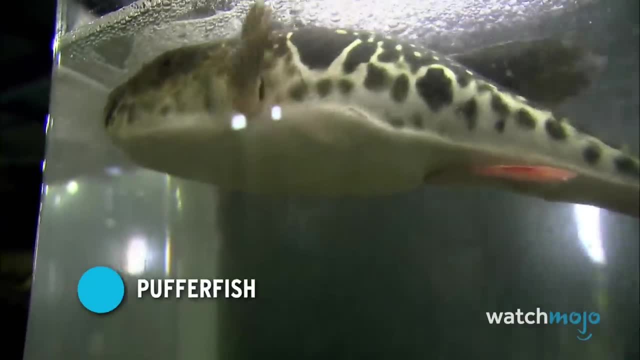 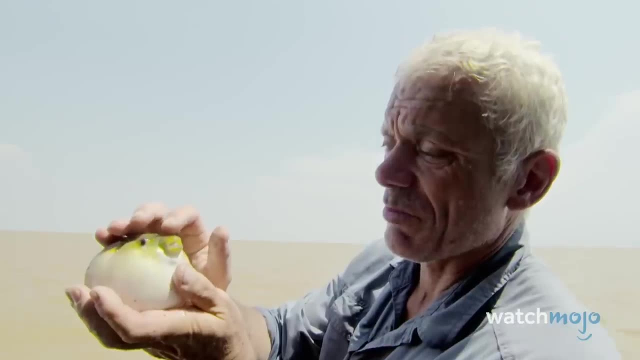 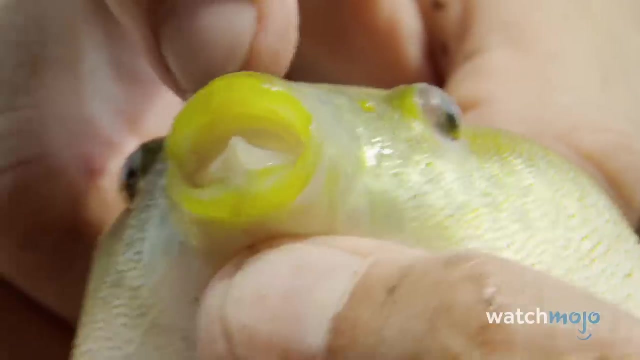 While not the biggest or most ferocious entry on our list, the pufferfish is nevertheless extremely dangerous. If inflating its body doesn't discourage predators, then its high levels of toxicity sure do. Just hoping it doesn't move suddenly. But I can see very clearly now those mouth parts. 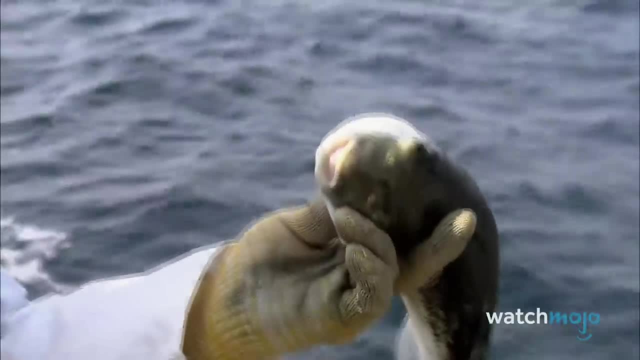 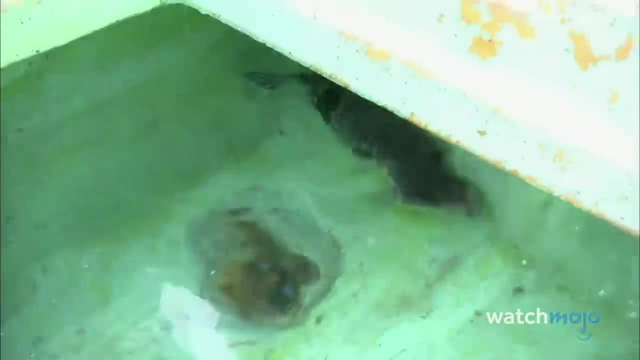 Pufferfish possesses a large amount of blood, which is why it's so dangerous. Pufferfish possess tetrodotoxin, which is over a thousand times more lethal than cyanide. A single pufferfish has enough tetrodotoxin to kill 30 adult humans. 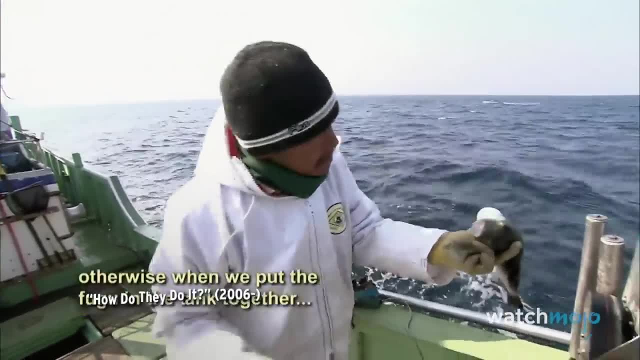 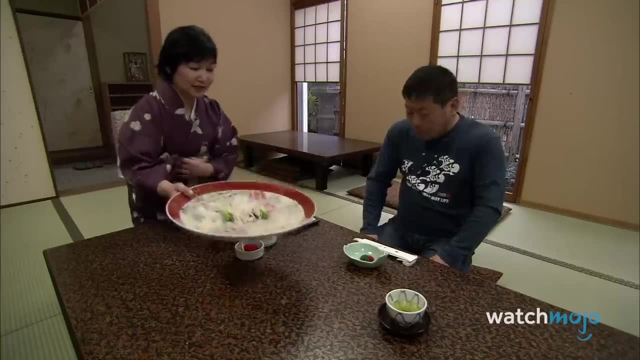 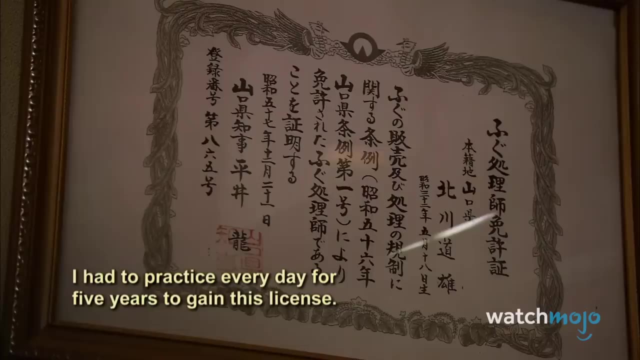 Pufferfish bite, So when you put it in your mouth you have to make sure it doesn't bite. In Japan, pufferfish, known as fugu, are considered a delicacy, But only licensed chefs are allowed to prepare it, as even the slightest mistake could prove fatal. 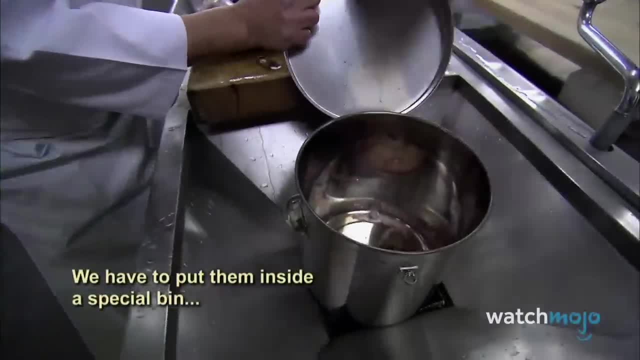 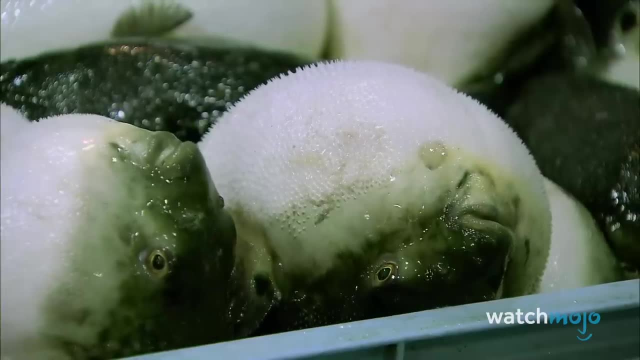 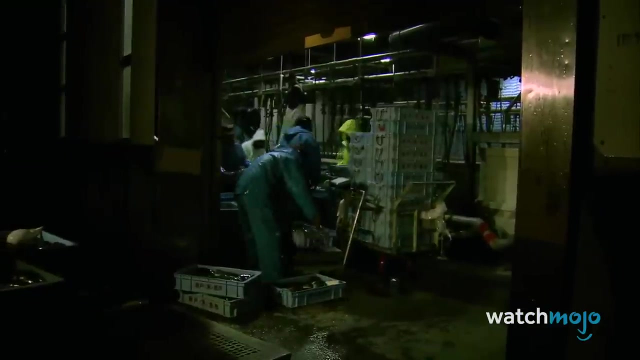 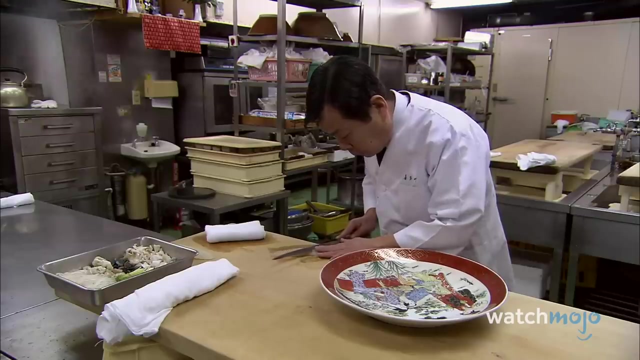 In 1958, the number of people who died from fugu poisoning peaked at 176, but has decreased over time, with about 20 fatalities being reported in Japan since the turn of the 21st century. To this day, no known antidote exists. 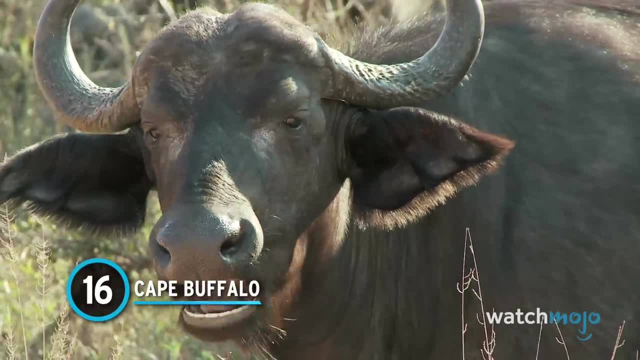 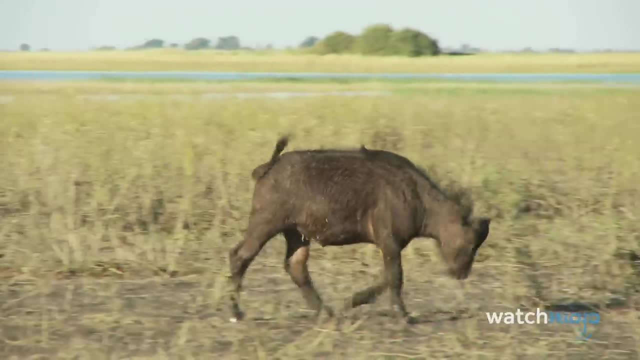 Number 16. Cape Buffalo. When you think of the most dangerous animals in Africa, the Cape Buffalo may not be your first or even fifth thought. They're responsible for hundreds of deaths every year, however, and eagerly go after jeeps and trucks, overturning them with ease. 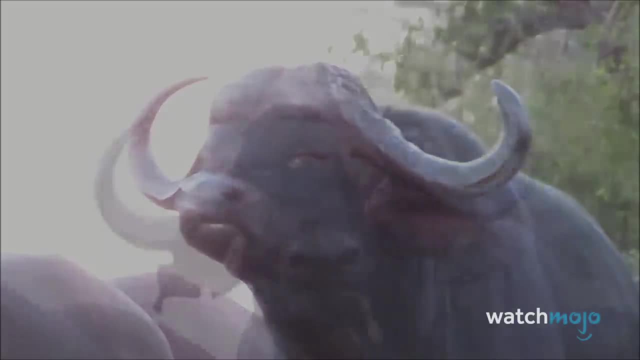 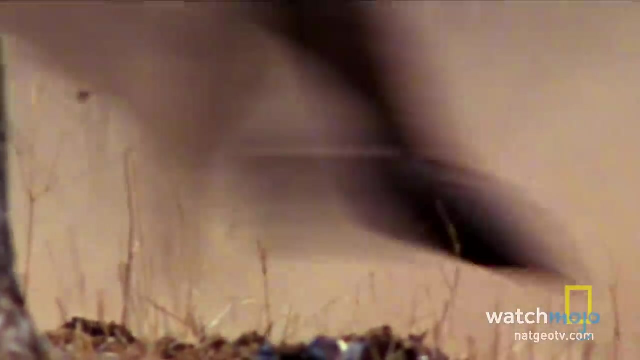 They're sometimes referred to as the Black Death and have been known to fight off crocodiles and lions. Their ability to run at 40 miles an hour, despite weighing 2,000 pounds, makes them one of the most dangerous animals in not only Africa but the entire world. 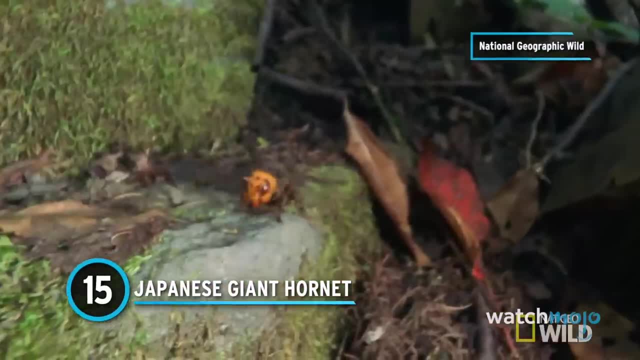 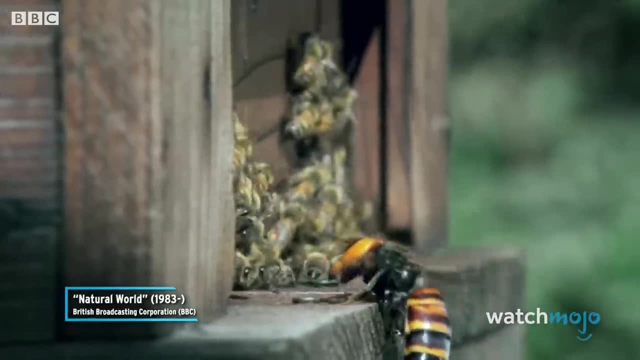 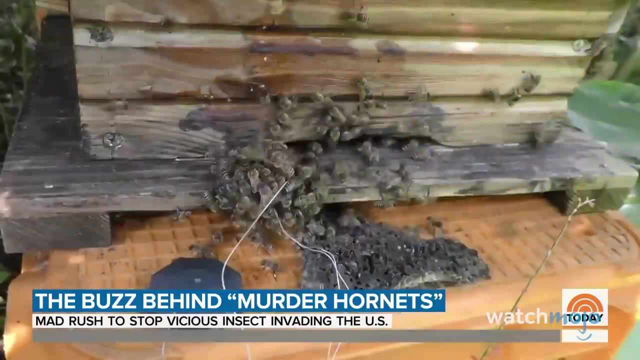 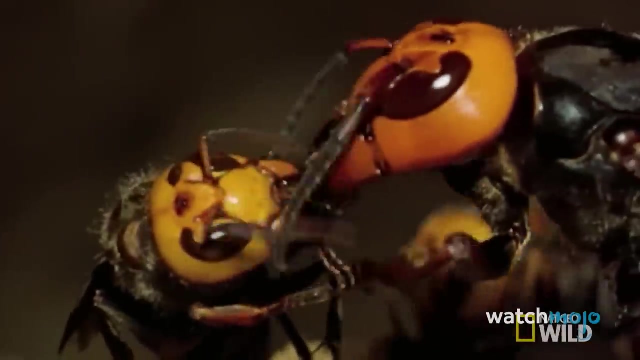 They're also known as the Japanese Giant Hornet. Afraid of bugs, Then these hornets are your worst nightmare. One by one, they're picked off, The largest of its kind on Earth. Japanese giant hornets are feared for their highly potent venom, which can kill a person if stung enough times, even if the venom doesn't kill right away. 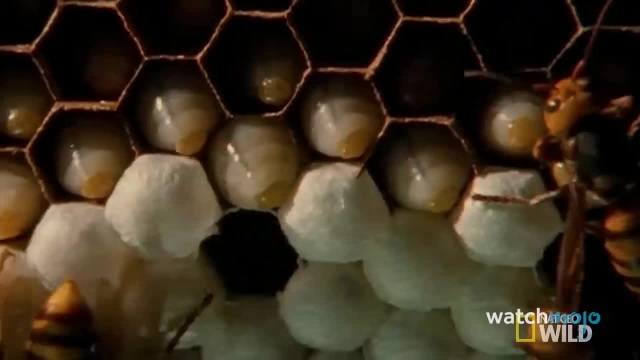 Those unfortunate enough to be stung by one are forced to endure intense, serious injuries to their body and mind. The Japanese giant hornet is known as the Japanese Giant Hornet and the most famous of its kind. They have been known for their high-dose venom, which is known to be the most deadly. 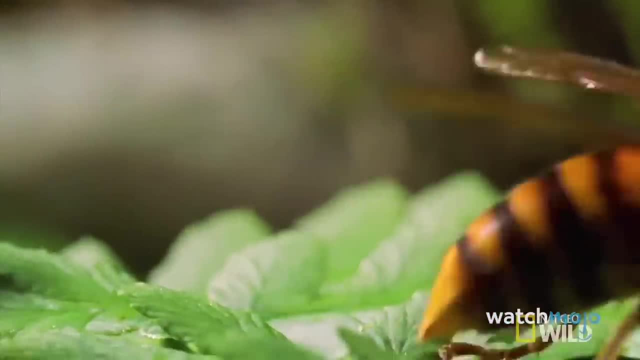 But even in the history of Japanese giant hornets. the Japanese giant hornet is known for its high-dose venom, which is known to kill very, very badly, hence searing pain. On average, these insects kill an estimated 10 to 50 people a year in Japan. 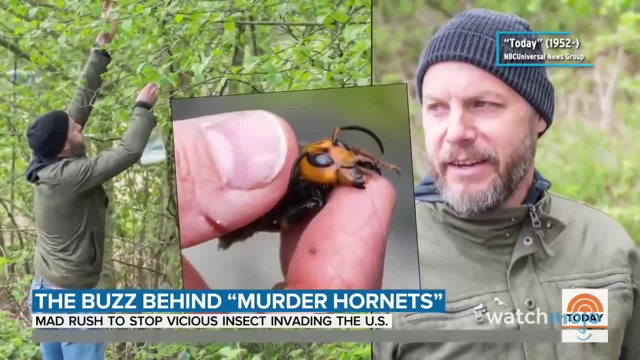 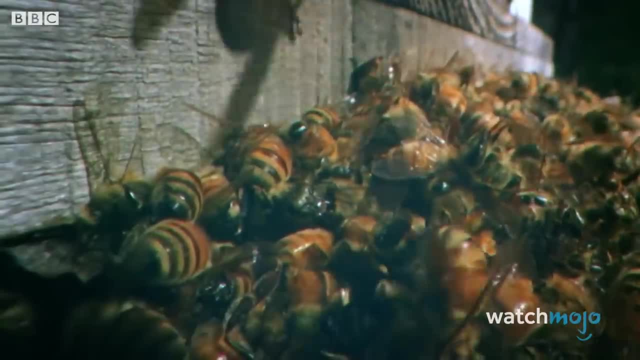 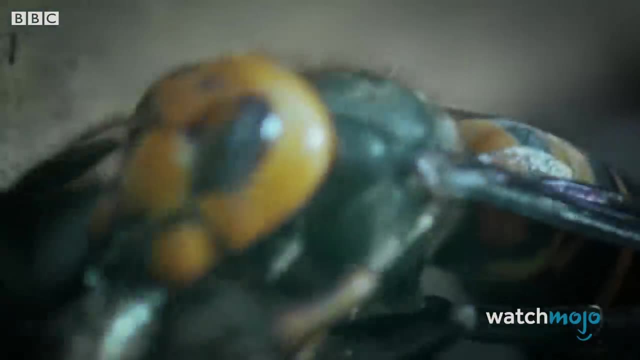 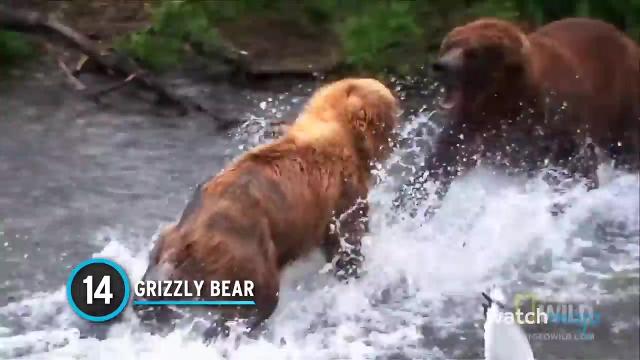 and injure many more. Recently spotted in the United States, this invasive species poses a significant threat to honeybee populations and the larger ecosystem. With such a terrifying reputation, it's no wonder they were given the nickname Murder Hornets Number 14.. Grizzly Bear Weighing between 400 to 800 pounds on average. 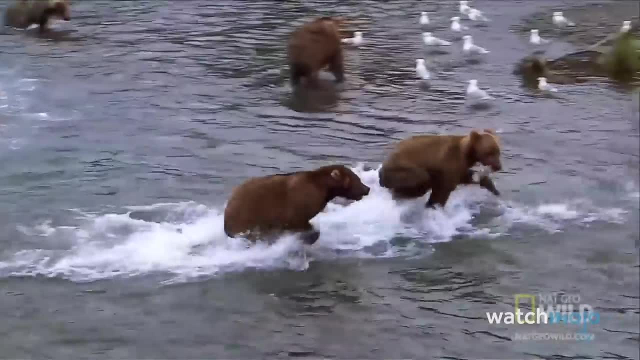 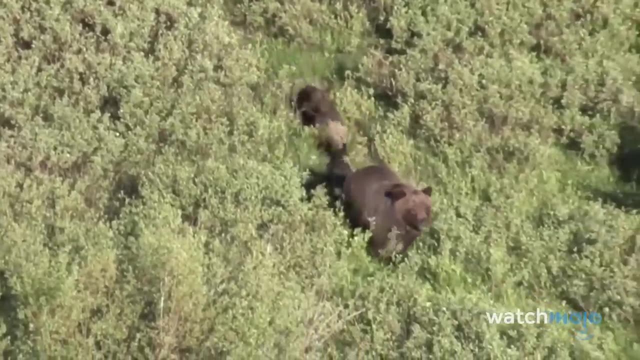 the grizzly bear is a force to be feared. While they may not actively hunt humans, urban expansion into their territory has made grizzlies more dangerous, as they've come to associate humans with food. While rare attacks from grizzlies are often fatal, 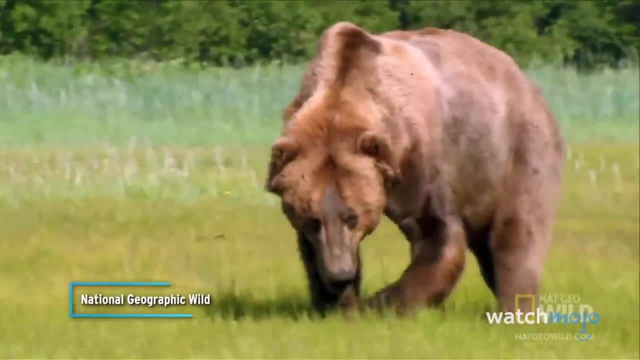 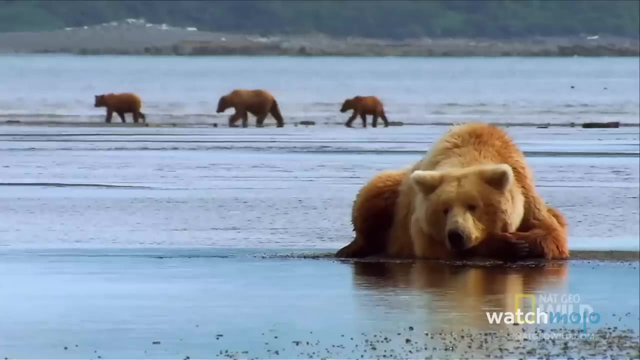 Mother Grizzlies. Mother grizzlies are especially dangerous as they can attack humans. They're more likely to attack if they feel their cubs are threatened. Along with their enhanced sense of smell and powerful claws, grizzlies can easily outrun humans and have a bite force strong enough to crush bowling balls. 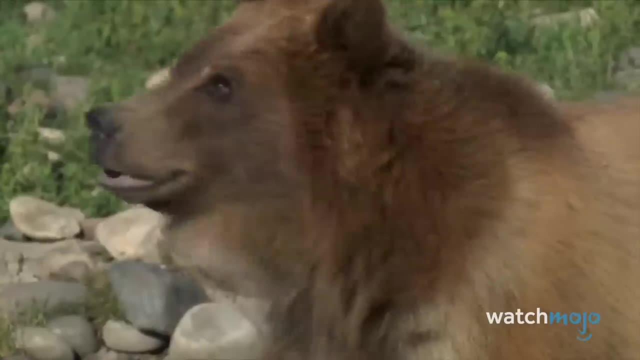 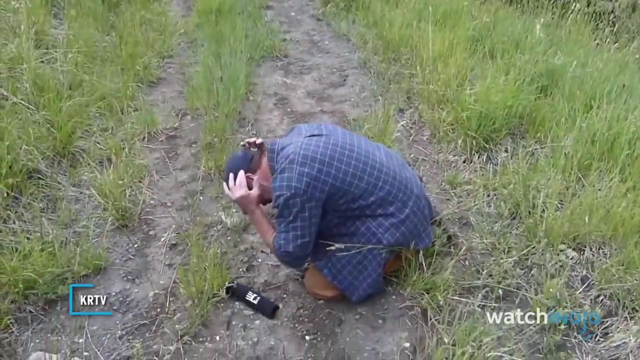 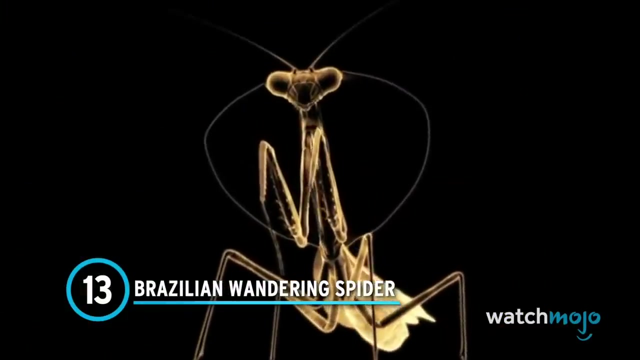 When heading out to grizzly country, knowing how to navigate an encounter with one could mean the difference between life and death. Number 13. Brazilian Wandering Spider. Unlike most spiders, this creepy crawly does not make its home in a web or lair. 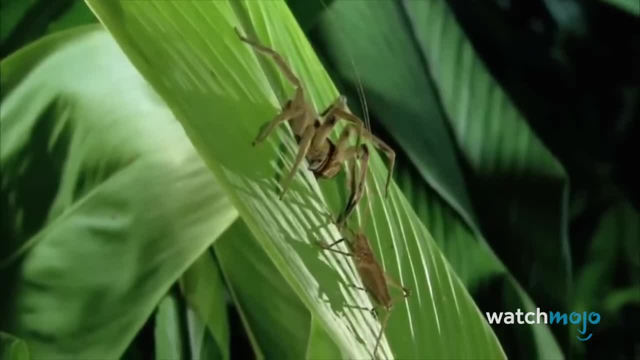 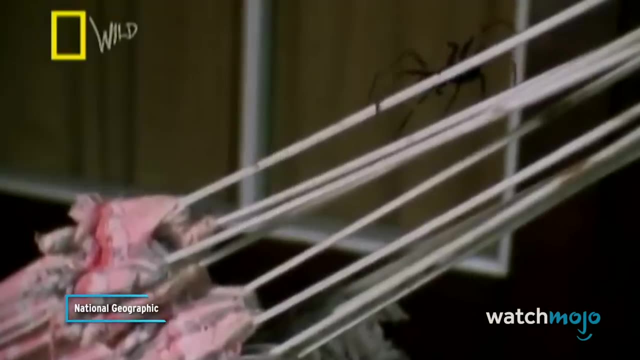 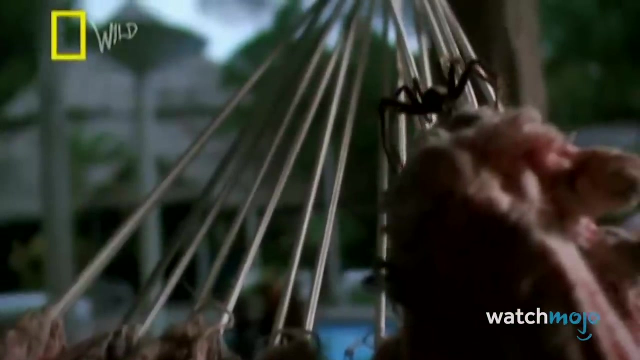 Rather, it lives a nomadic lifestyle, hunting and ambushing its prey. This makes the Brazilian Wandering Spider even more dangerous, as it often wanders into human settlements Known for hiding in dark places such as boots and shoes. these spiders thus bite people in self-defense. 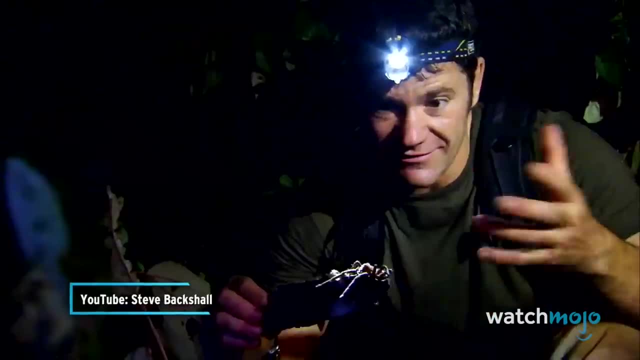 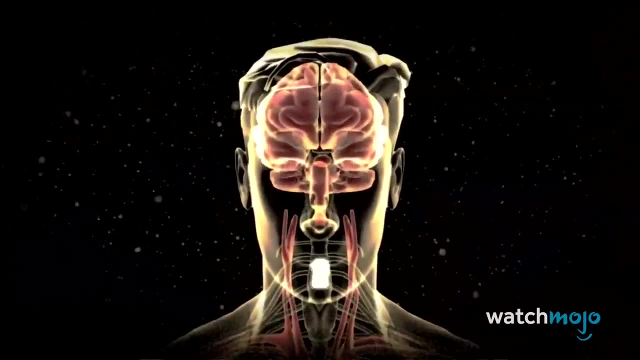 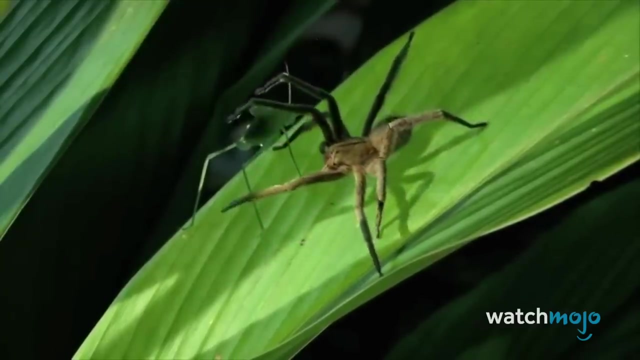 Afterwards, it can result in a total destruction of someone's sex life for the rest of their life. While its venom can be treated with anti-venom, it is still the most potent poison of any spider. It directly targets the nervous system, which can potentially be fatal, making it extremely dangerous, especially for children. 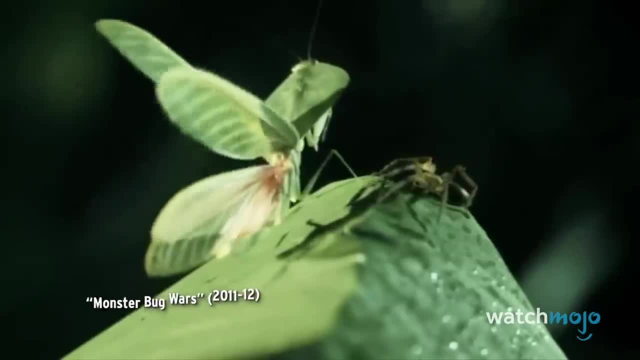 Number 14. Spotted Spider. We'd expect nothing less from a spider who's very dangerous. We'd expect nothing less from a spider who's very dangerous, especially for children. We'd expect nothing less from a spider who's very dangerous, especially for children. 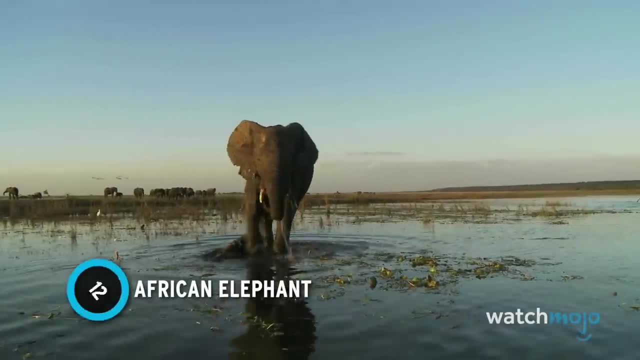 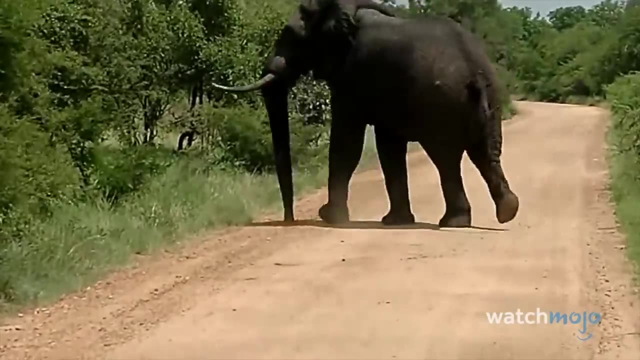 The word genus translates to murderous Number 12.. African Elephant. Elephants are one of the most popular creatures on the planet, but that doesn't make them any less dangerous. They've been known to become extremely aggressive without warning, making them one of the more unpredictable animals on the planet. 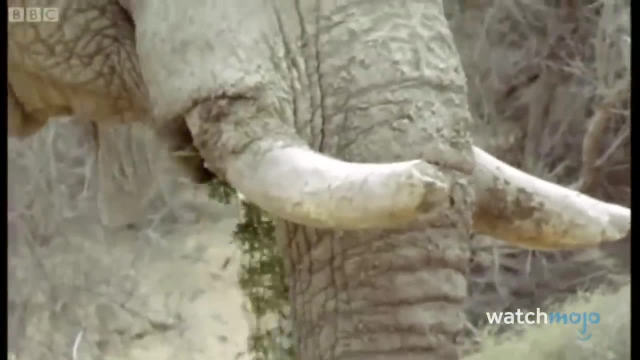 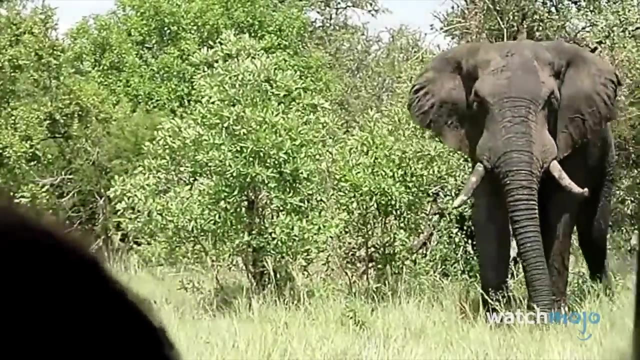 This is especially dangerous because they frequently come into contact with people through safaris and other ventures. It seems like at least once a year there is a story about an elephant wandering into a village and trampling dozens of people, trampling dozens of people. 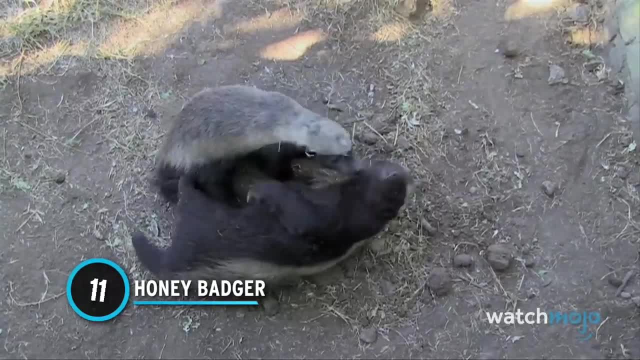 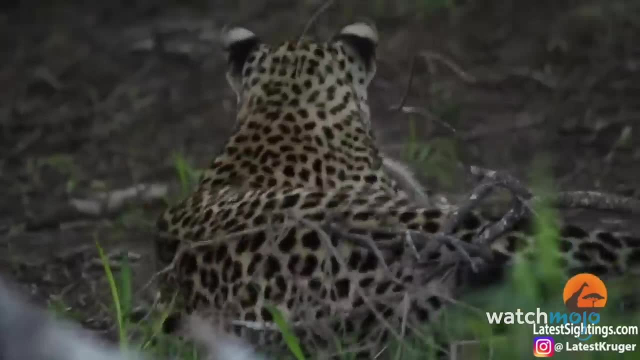 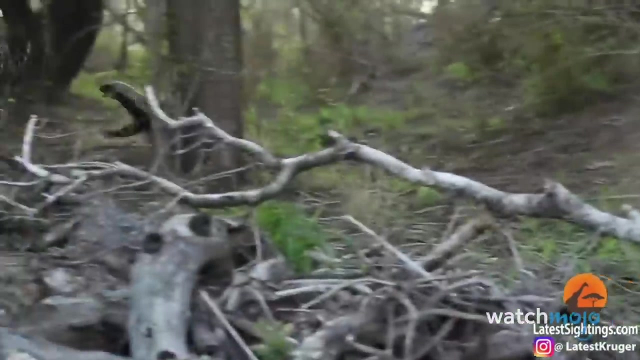 Considered the most fearless animal alive by the Guinness Book of World Records, the honey badger is one of nature's most relentless hunters. It possesses powerful claws and fangs that can break open tortoise shells. It also has a strong resistance to venom and a loose but thick hide. 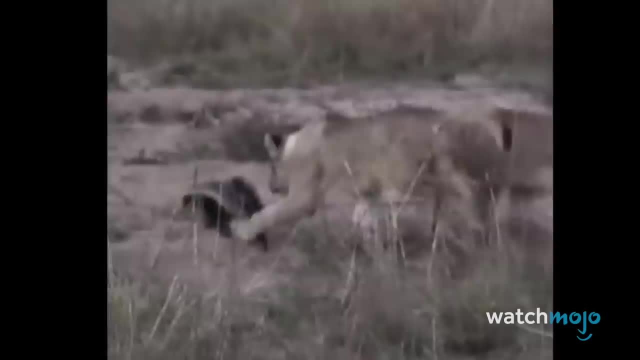 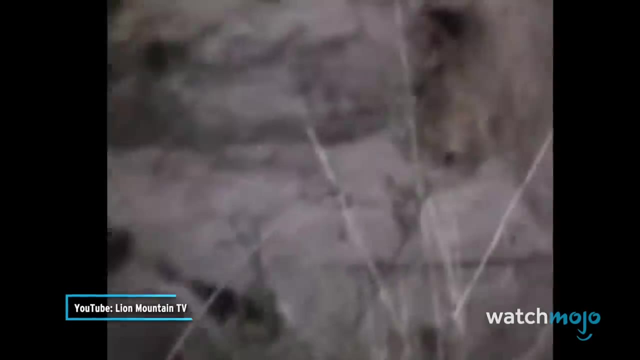 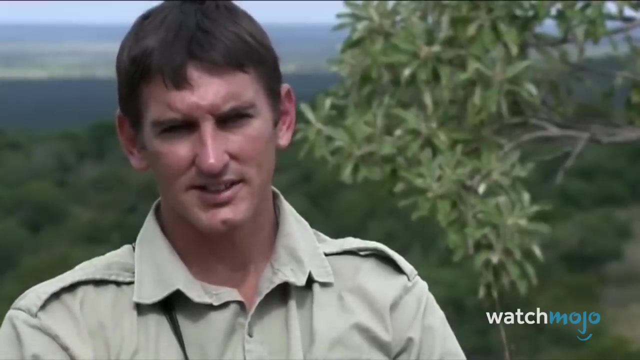 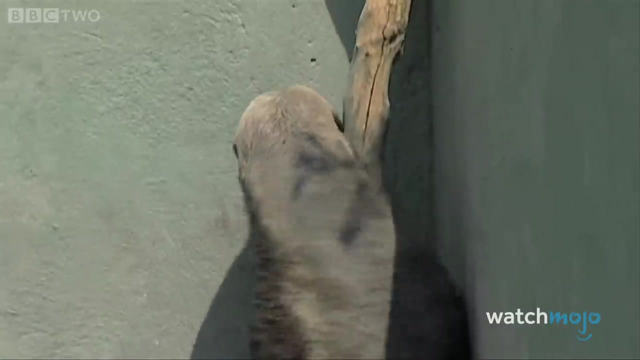 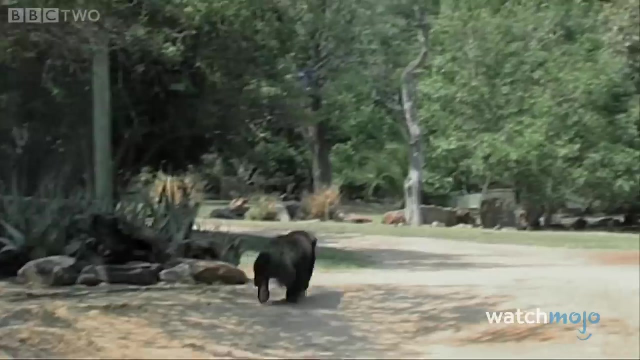 tough enough to resist blows from a machete, The honey badger won't hesitate to challenge and even repel much larger predators such as leopards and lions. They're also highly intelligent or can escape from or break into secure enclosures. Because they often attack livestock and bee farms, they increasingly get into conflicts with humans. 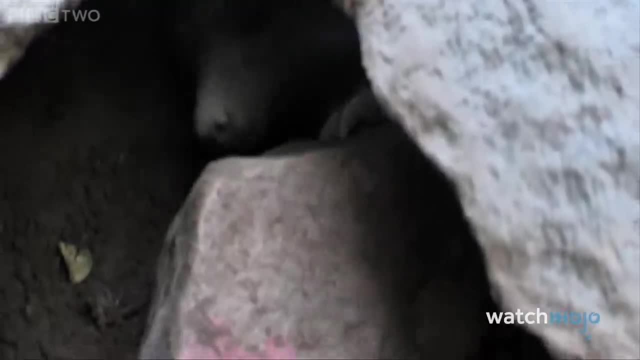 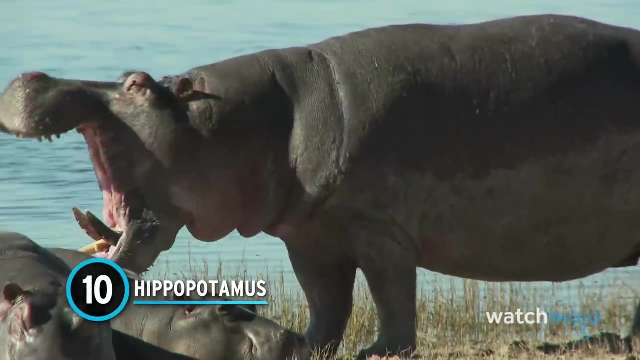 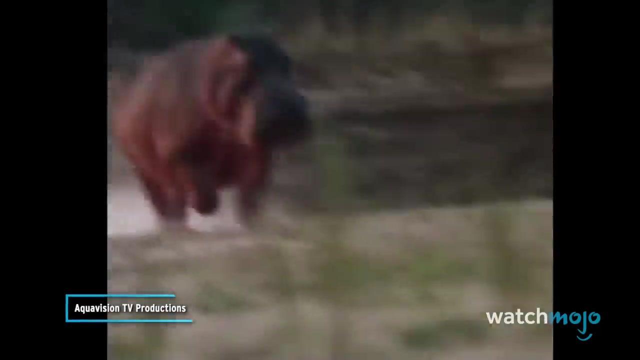 When provoked, they are terrifying and will fight to the death if escape is impossible. Honey badger, don't care. Number 10. Hippopotamus. While hippos may not necessarily come across as an extremely dangerous animal, they are aggressive and have been known to attack people without provocation. 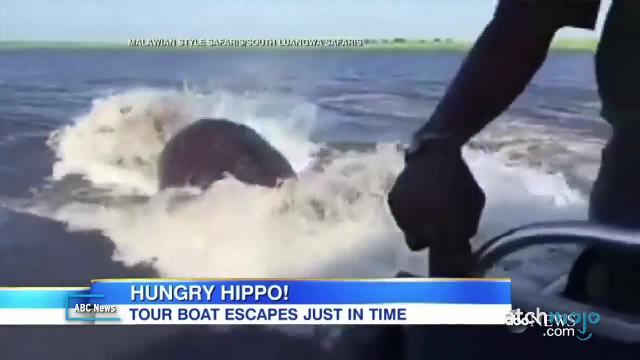 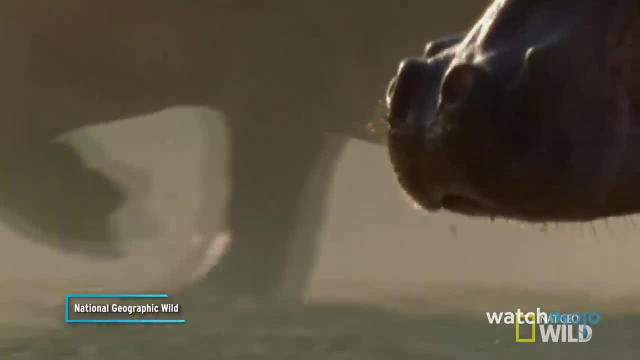 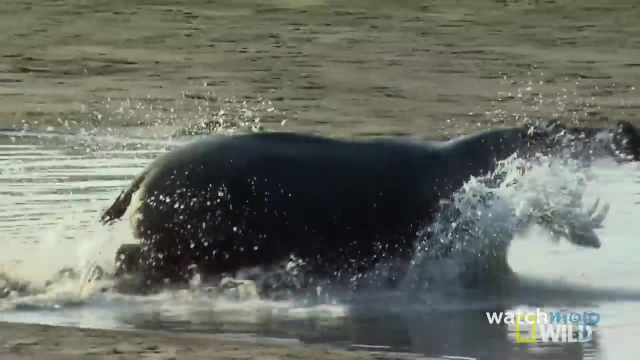 They are usually found in Africa and are one of the larger animals responsible for killing the most humans on that continent. Despite weighing several thousand pounds, a hippo can run as fast as 20 miles per hour and has an extremely powerful mouth. They can decimate safari vehicles without breaking a sweat. 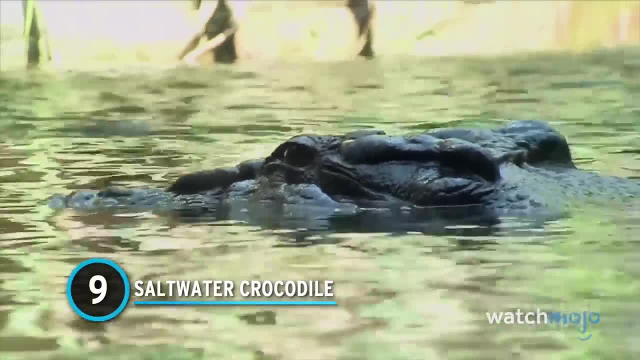 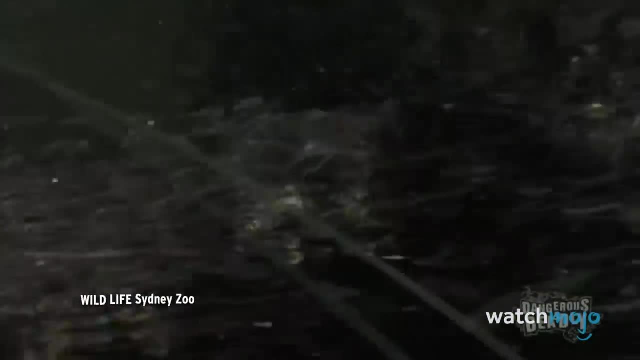 Number 9. Saltwater Crocodile, The largest reptile in the world. saltwater crocodiles are extremely dangerous and are responsible for attacking hundreds of people every year. They are found all over the world in all sorts of habitats, including both saltwater and freshwater. 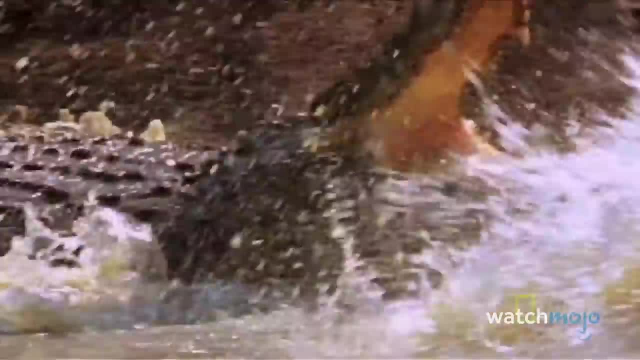 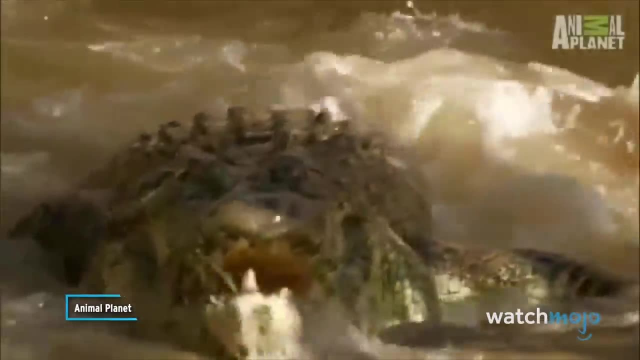 They have the strongest bite of any animal currently in existence, with their jaws capable of applying over 3,500 pounds of pressure per square inch. They have an alarming tendency to consider humans as their prey, although only if we venture into their territory. 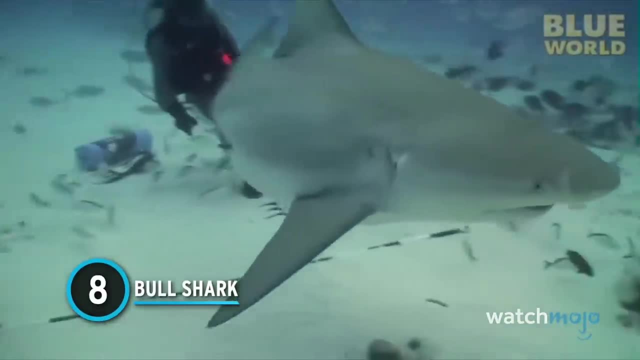 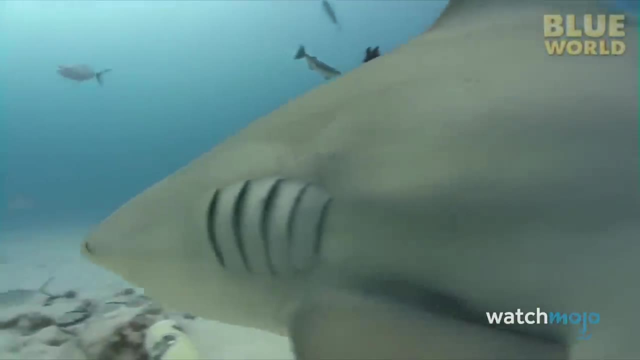 Number 8. Bull shark. Alongside great white and tiger sharks, the bull shark is one of three shark species most likely to attack humans unprovoked, While the great white has been implicated in more unprovoked attacks on humans. several factors make the bull shark more. 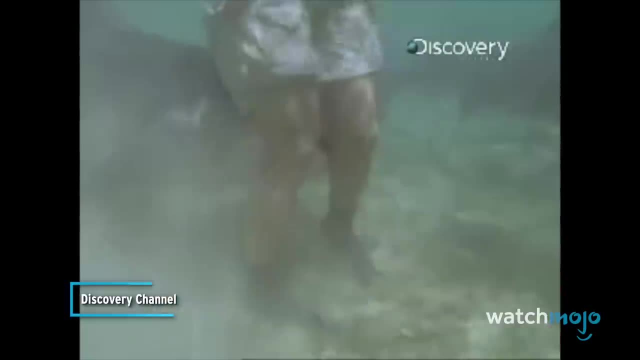 dangerous to humans than any other shark species. Number 1. Bull shark. The bite was in the calf. It was Number 1. Bull shark, just like us. Number 1. Bull shark is more dangerous to humans than any other shark species. 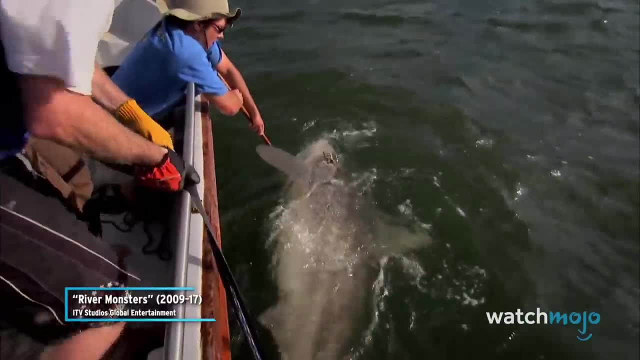 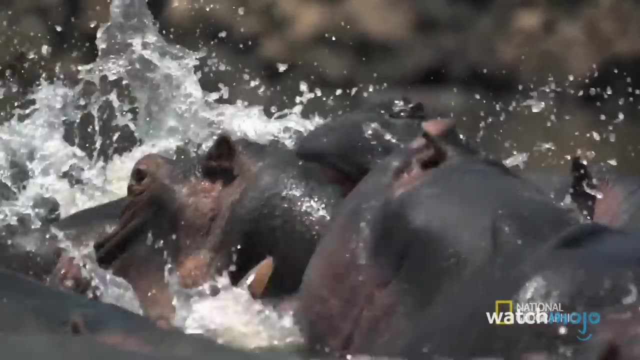 Number 1.. Bull shark is more dangerous to humans than any other shark species. These include its high aggression level, a much more powerful bite force than the great white and, most dangerous of all, its ability to thrive in both saltwater and freshwater sources. 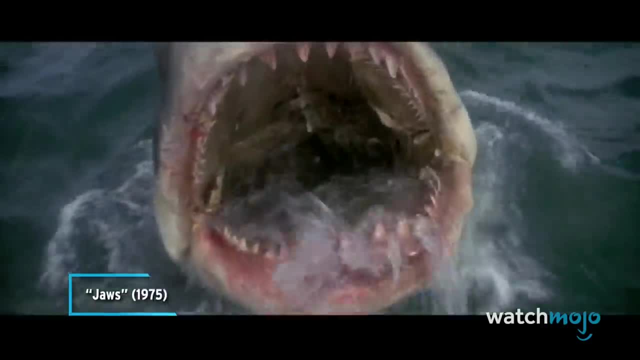 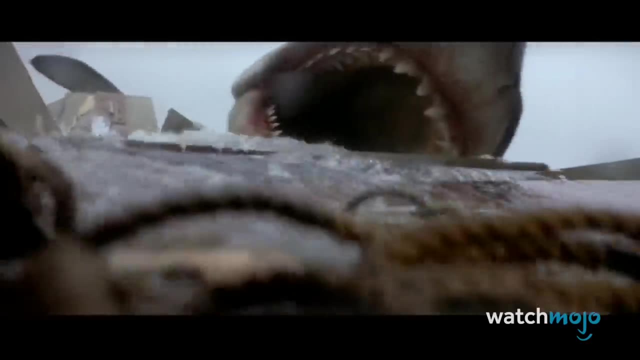 In rare cases, bull sharks have even been sighted going far up both the Mississippi and Ohio rivers. Some experts believe that the bull shark was responsible for the Jersey Shore attacks of 1916, an event that inspired the novel Jaws Number 7.. Sloth bear. 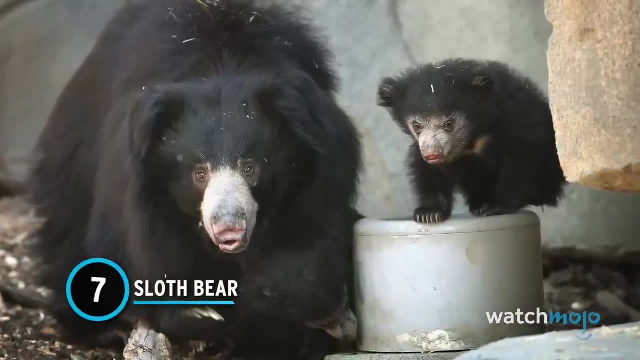 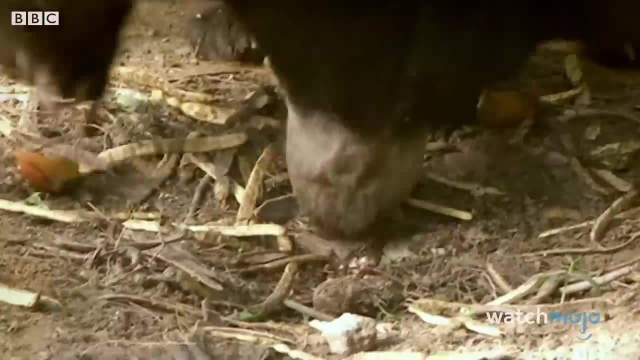 Native to the Indian subcontinent. sloth bears may look adorable and fluffy, but they're extremely aggressive. They have a reputation for regularly attacking humans more than any other bear Number 1. Sloth bear- Those would be in the wild, used for just this purpose, but mostly for digging into termite. 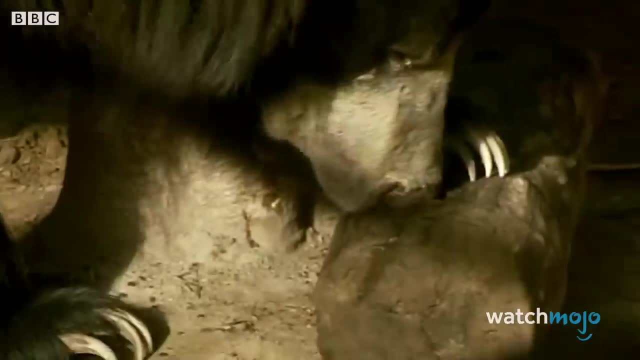 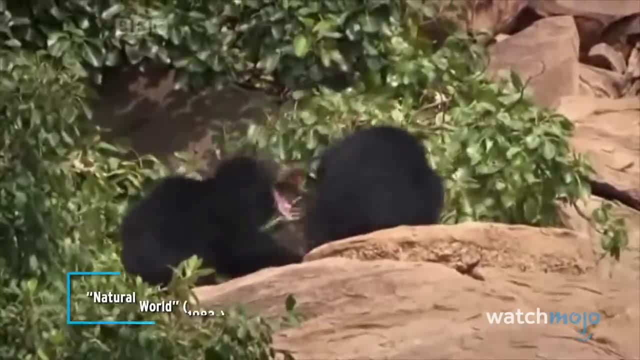 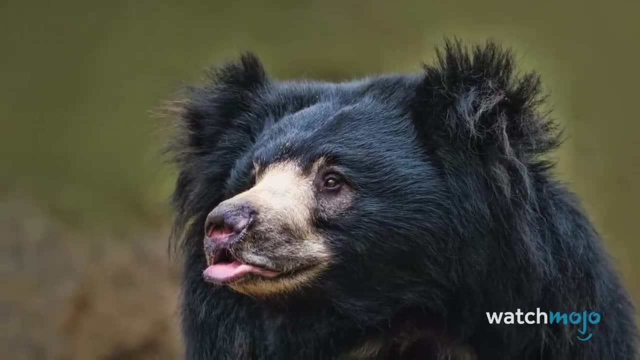 Number 1. Sloth bear. Number 1. Sloth bear increased as the animals wander into towns in search of food. Due to their poor eyesight, sloth bears are easily startled and thus more likely to lash out in self-defense or to defend their cubs. 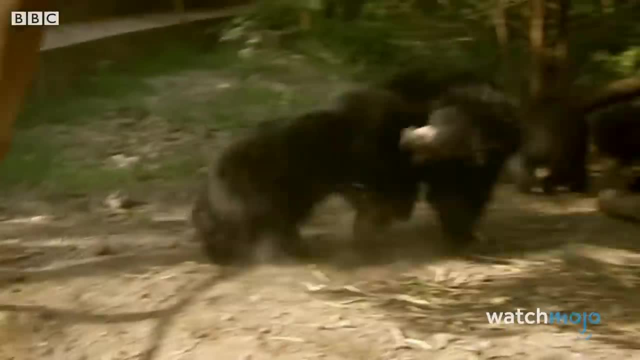 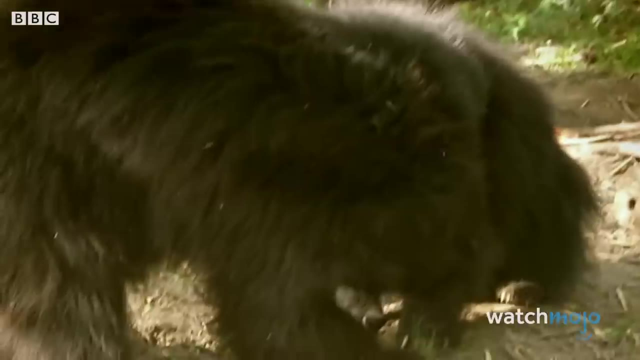 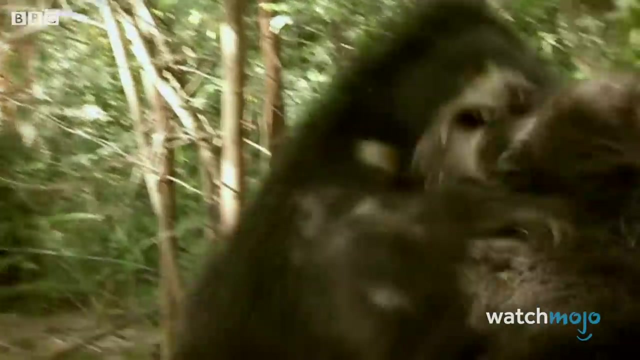 Between 1998 and 2000,. 137 sloth bear attacks, including 11 fatalities, occurred in the North Bilaspur Forest Division in the state of Chhattisgarh. In 1957, a specimen known as the sloth bear of Mysore achieved notoriety for killing at 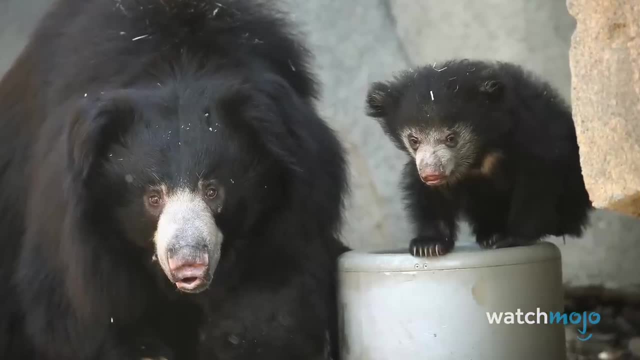 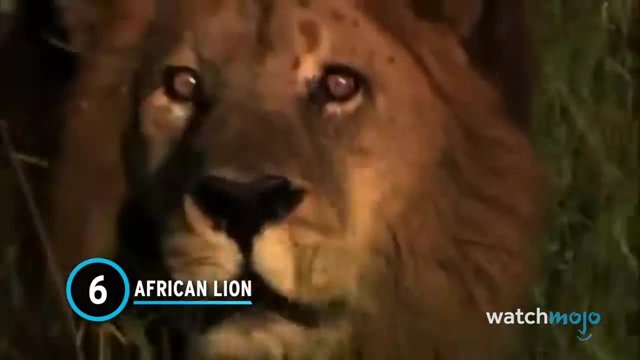 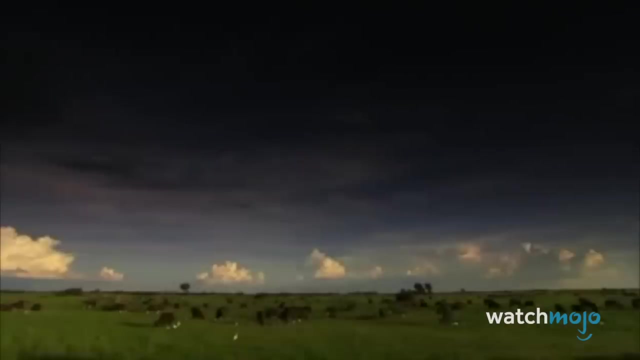 least 12 people and seriously injuring over 20 others. Take one look at an African lion and you know that you are putting your life at risk just by getting within striking distance of the animal. This doesn't seem to stop humans from going on safaris or attempting to tame them, however. 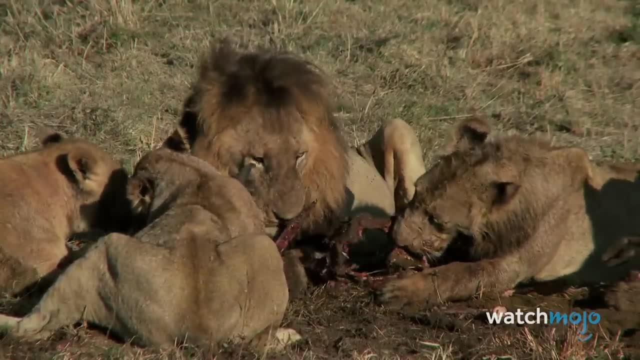 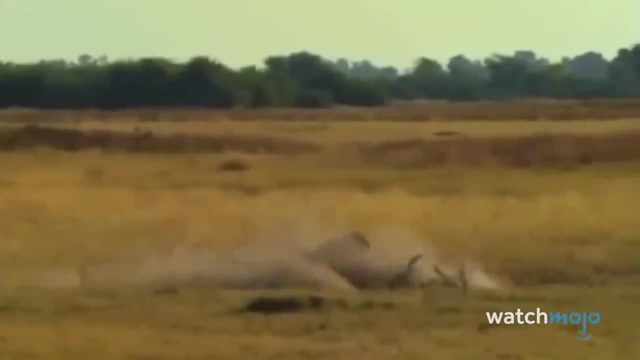 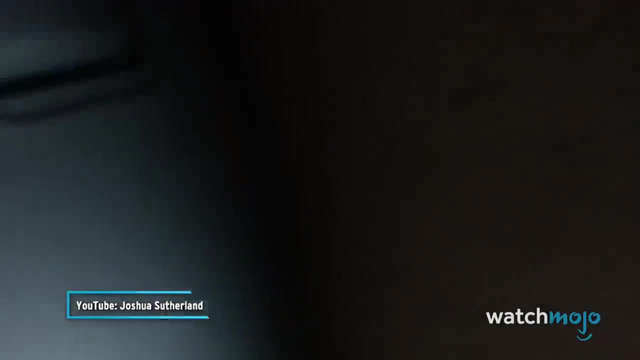 Hundreds of people die every year at the hands of the African lion. Luckily, they do not actively seek out humans, but their amazing speed and razor-sharp teeth and claws mean that if they do decide to make you their prey, you are in a lot of trouble. 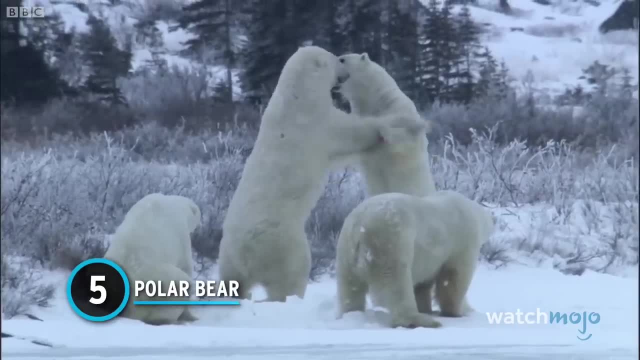 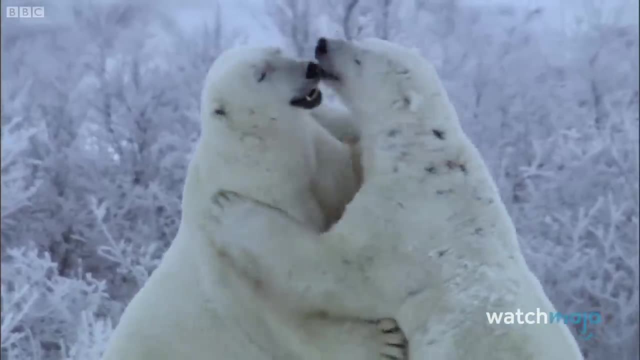 Number 5. Polar Bear. Raised in the harsh environment of the Arctic Circle, polar bears have evolved into one of the world's apex predators. Reaching heights of more than 9 feet and weighing over 1,000 pounds, polar bears are the most. 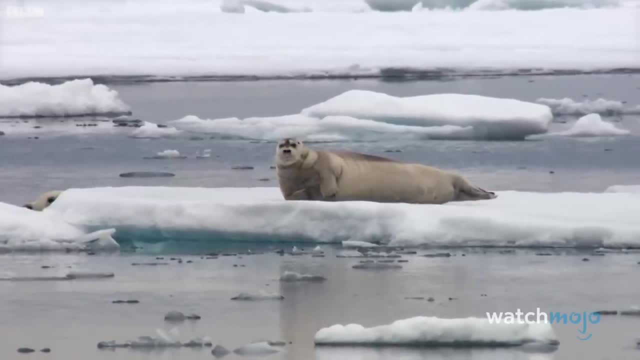 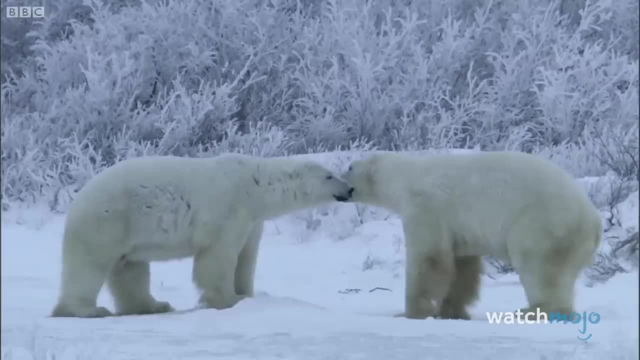 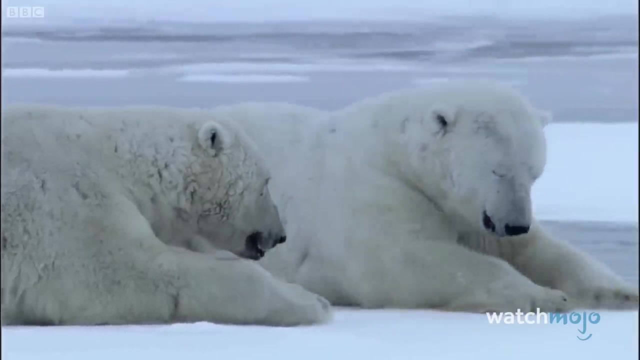 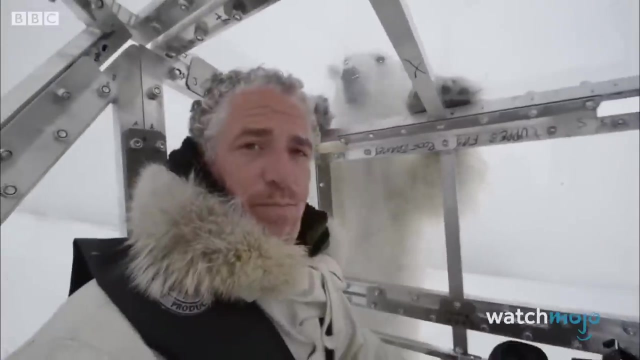 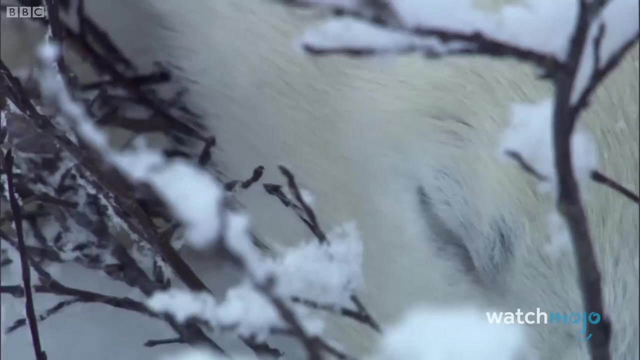 powerful carnivores on Earth. While normally cautious by nature, hungry polar bears will kill and eat virtually anything big or small, including humans. with the loss of their habitat due to climate change and fear towards people, more and more polar bears are drawn towards human populations in search. 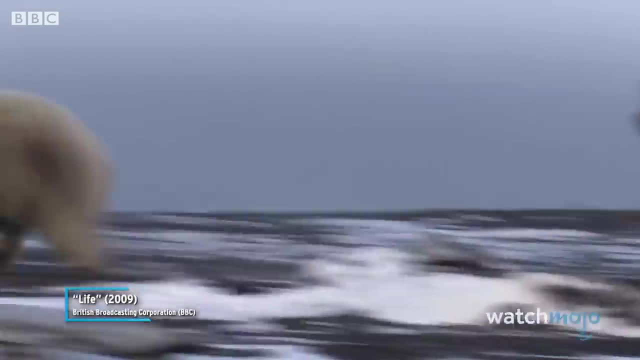 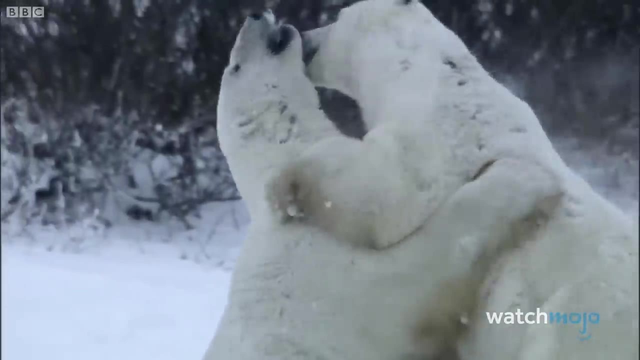 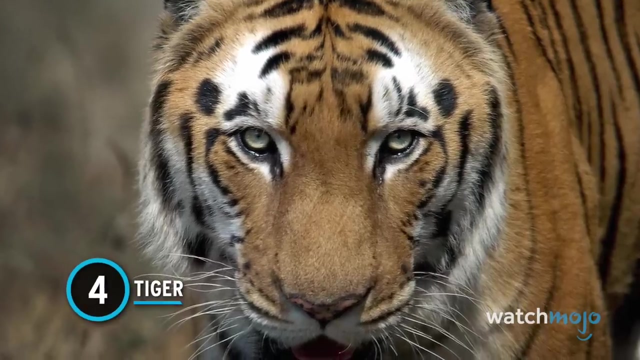 of food. Given the polar bear's immense size, powerful claws and teeth, capable of tearing a human to shreds, any encounter can prove fatal. Number 4. Tiger. As one of the world's most iconic animals, the tiger has left its mark in history, mythology and popular culture. Number 5.. Tiger is the biggest predator of all time, Along with being the largest cat species. tigers can be divided into several subspecies, such as the common Bengal tiger and the Siberian tiger, With jaws strong enough to crush the throats of its prey, and paws capable of inflicting. 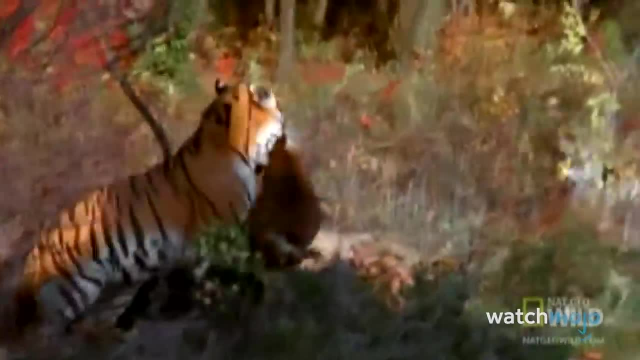 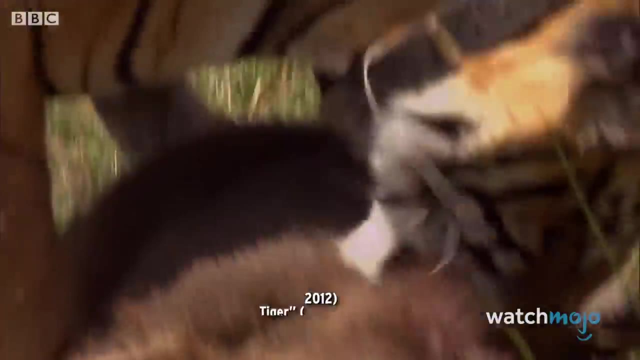 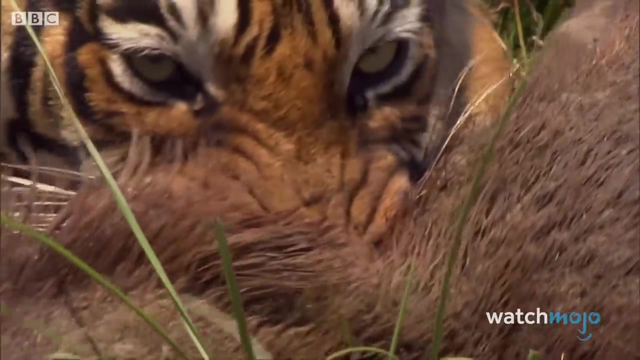 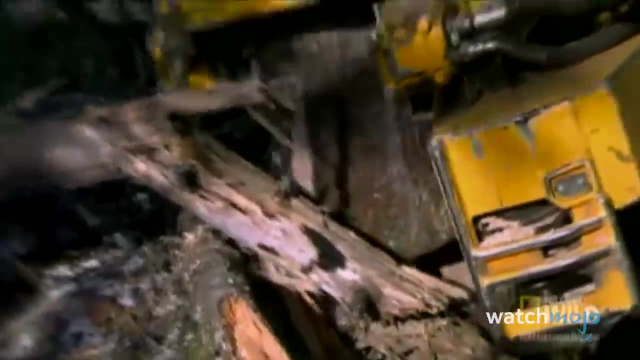 heavy blows. tigers are apex predators that are praised and feared for their legendary strength and hunting prowess. Number 6. Chumpawut Tiger. Some tigers have even acquired a fearsome reputation for being man-eaters, with the most infamous being the Chumpawut tiger, which allegedly 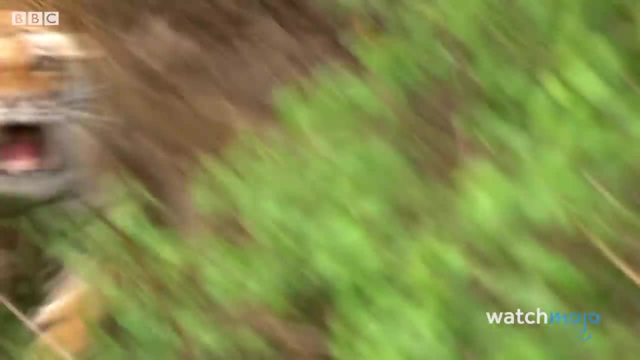 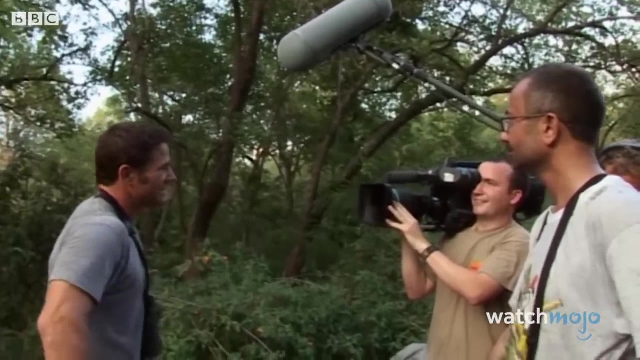 killed more than 400 people over the course of seven years at the turn of the 20th century. Number 7. Chumpawut Tiger. I could see Johnny the cameraman nearly jumping out of his skin, and you're sweating a fair bit there, Johnny. 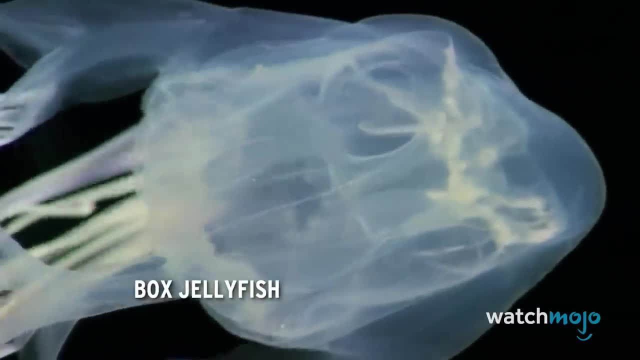 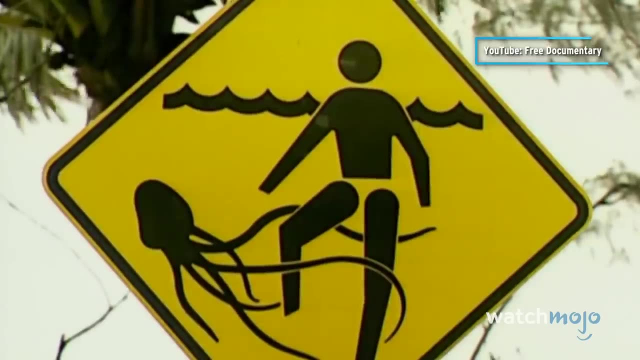 Anyway, I thought it was a car. Anyway, I thought it was a car at one point. Number 3. Box Jellyfish: If you come across one of these creatures while scuba diving or floating in the sea, get away as fast as possible. 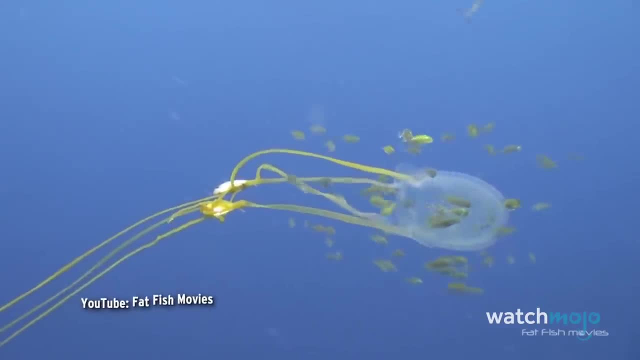 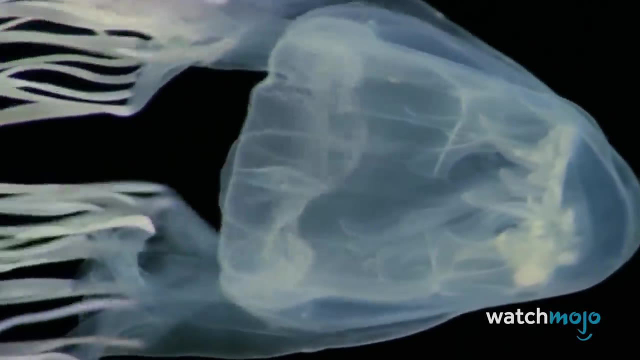 The box. jellyfish is one of the most venomous animals on the entire planet, a category that includes frogs, scorpions and snakes. It can possess as many as 60 tentacles, and their sting can kill a human, either by paralyzing. 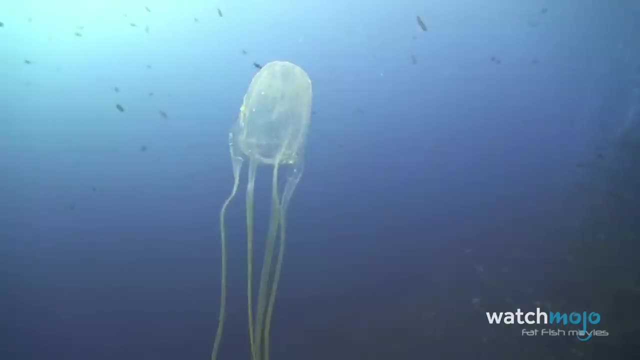 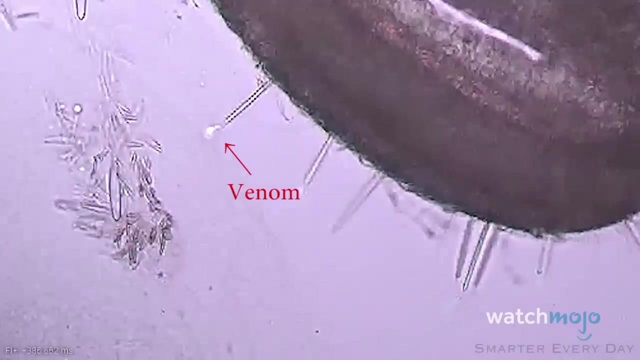 them, which leads to drowning or by stopping their heart. Luckily, many people survive encounters with the box jellyfish, but not without first experiencing excruciating pain. Number 2. Black Mamba Snake, Despite being the second most venomous snake. 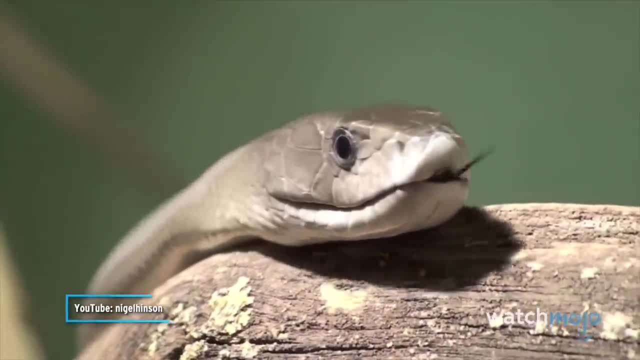 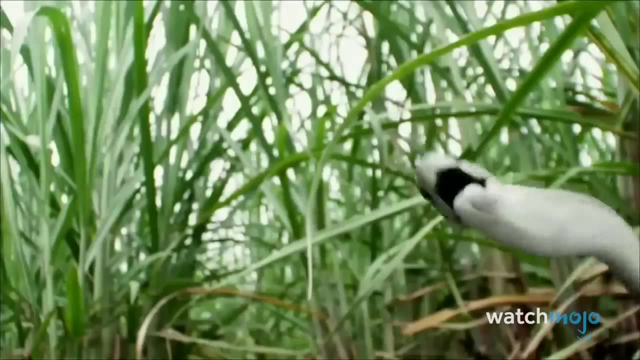 in the world. the black mamba makes our list because it is the most feared snake in all of Africa, which is saying something. Their bite has been called the kiss of death and it can kill a human in less than 10 hours if not treated effectively. 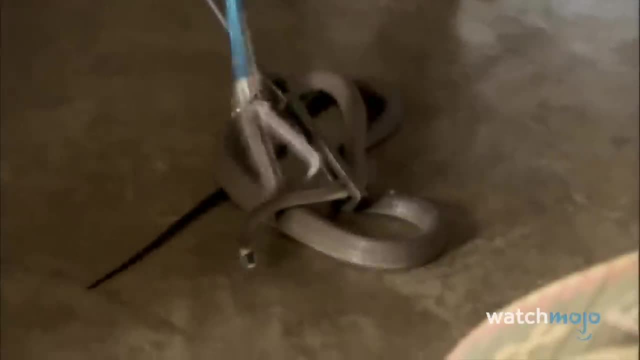 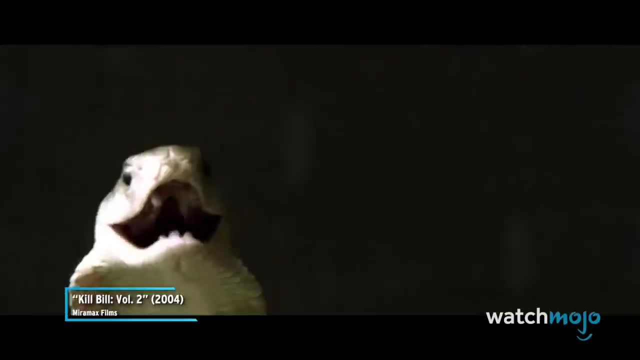 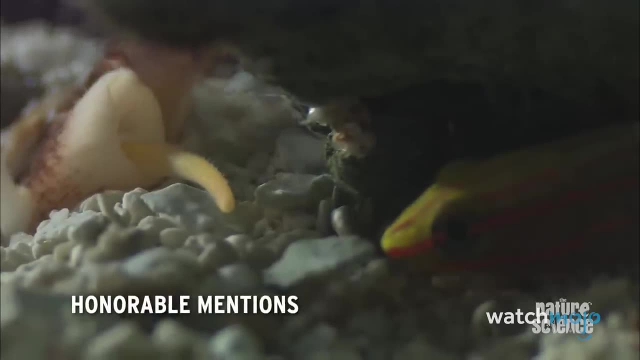 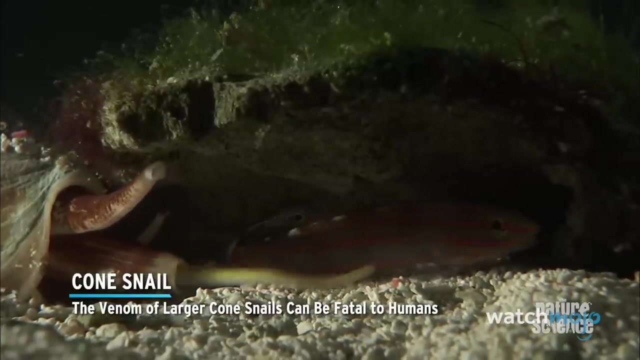 If they attack with their weapons. they will attack if they feel threatened, delivering deadly strikes in rapid succession. Number 1. Cone Snail. Before we unveil our number one pick, here are some honorable mentions. Cone Snail, The venom of larger cone snails, can be fatal to humans. 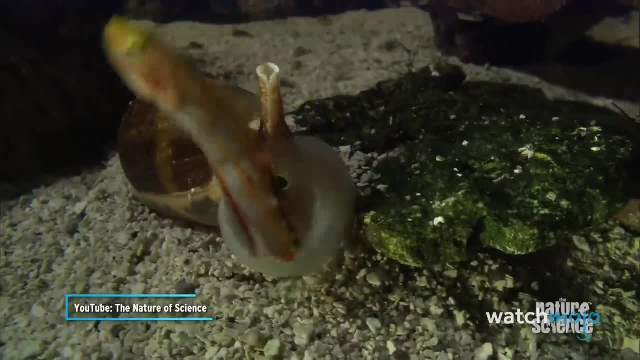 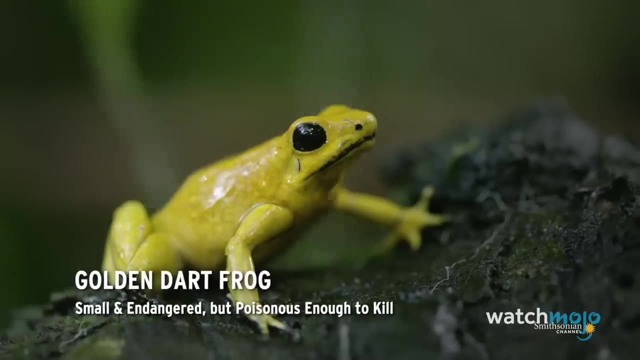 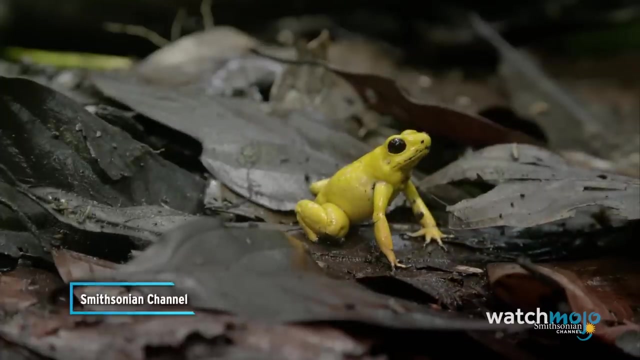 Injects it with venom, causes paralysis within one or two seconds. and then they hauled in like a fishing line down their throat into their stomach. Golden Dart Frog, small and endangered, but poisonous enough to kill Komodo Dragon, the world's largest lizard. 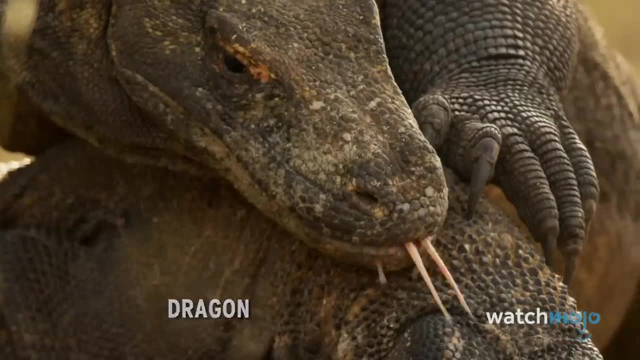 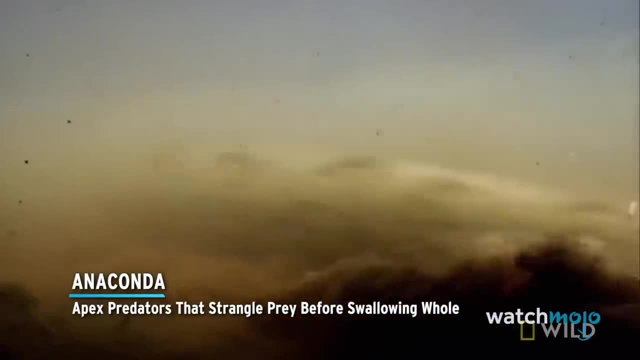 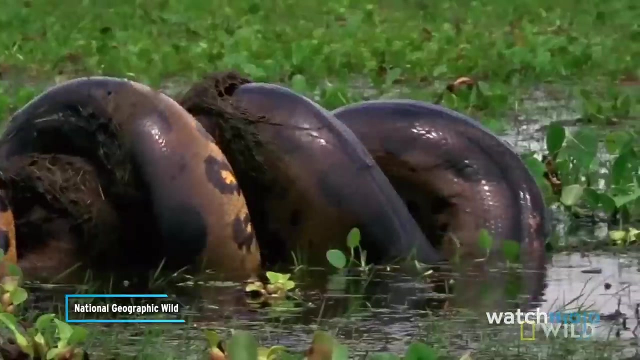 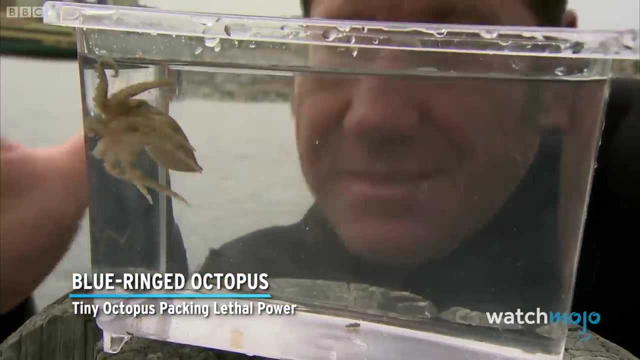 with a toxic bite In dragon society. size is everything: Anaconda, apex, predators that strangle prey before swallowing whole. It strikes, latching on with six rows of teeth, coiling itself around the large rodent. Blue-ringed Octopus, tiny octopus, packing lethal power. 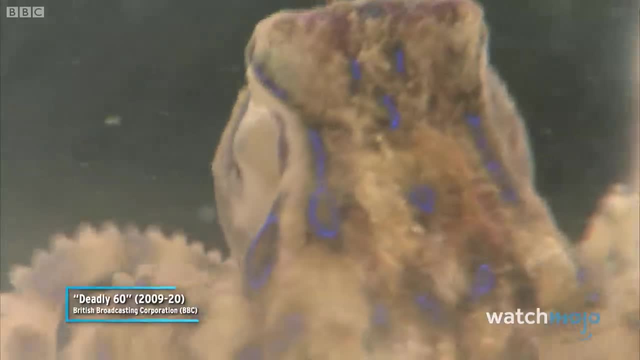 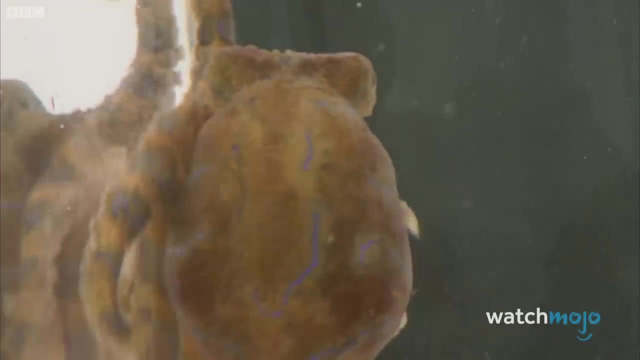 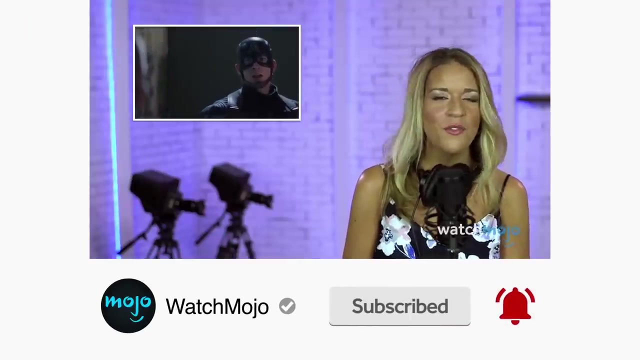 And you should see the plainly colored animal take on incredible agitated colors: bright, neon, blue circles. Look at that, Wow. Before we continue, be sure to subscribe to our channel and ring the bell to get notified about our latest videos. You have the option to be notified for occasional videos.